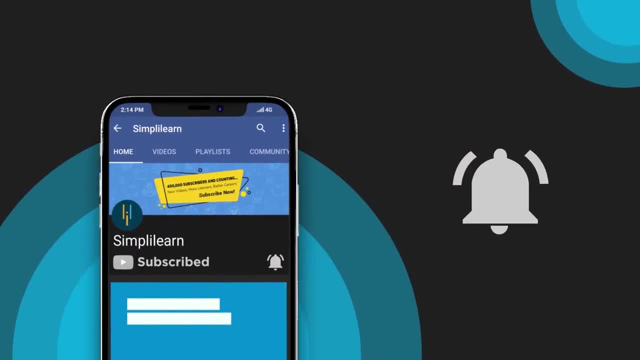 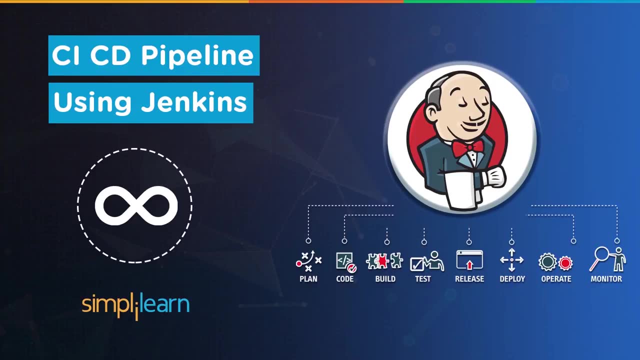 Welcome everyone to another topic on CICD pipeline using Jenkins. Now, in this one, we are going to talk about that: how exactly we can go for a CICD implementation with a pipeline concept, and that, too, with the help of Jenkins tool. So let's talk about what exactly we are going to talk about Now. 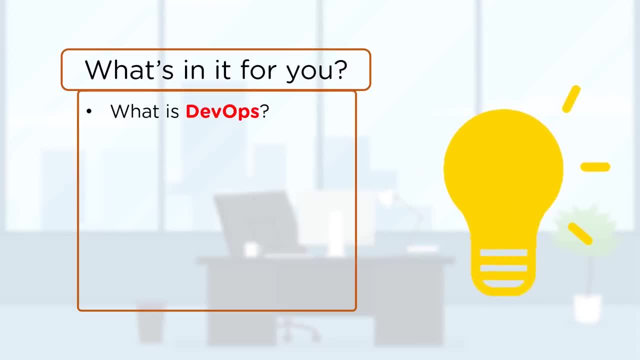 first of all, we are going to talk about like what exactly is in DevOps process, and then we are going to talk about like what is the importance of CICD pipeline. Then we are going to take care of a kind of a sample pipeline, which is there a kind of a building a CICD pipeline, with the help of Jenkins. 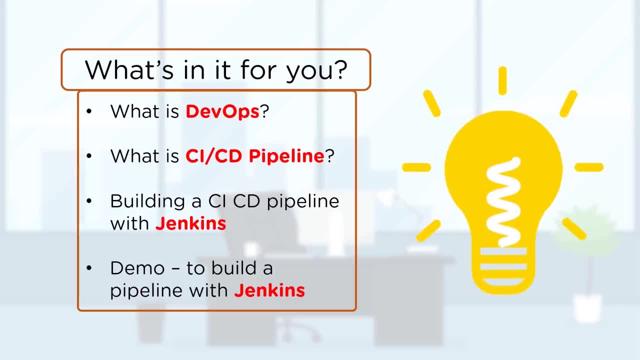 here And in the end we are going to see a small demo on how we can do this setup so that we can have some particular pipeline process and executed and processed all together. So let's talk about the different things one by one Now. the first one is that what exactly is in DevOps here Now? 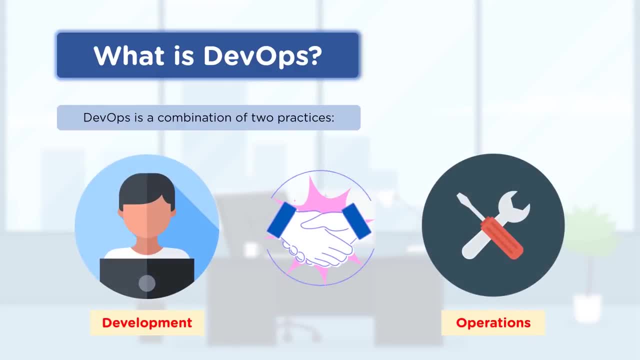 DevOps is basically a combination of two practices, Like that is, the development- and operations. So development is having their own task of doing the development and preparing the source code, and operation is responsible for deploying the source code to a specific environment, whether it's a production or any. you know other environment. 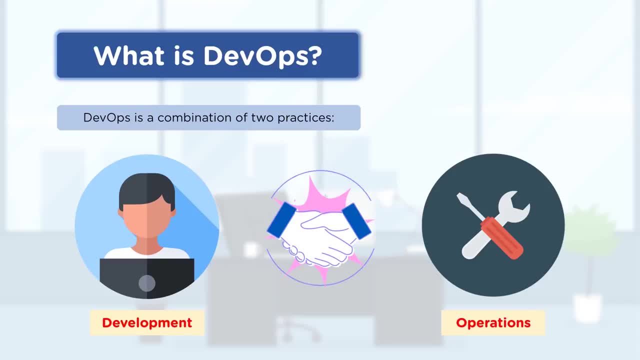 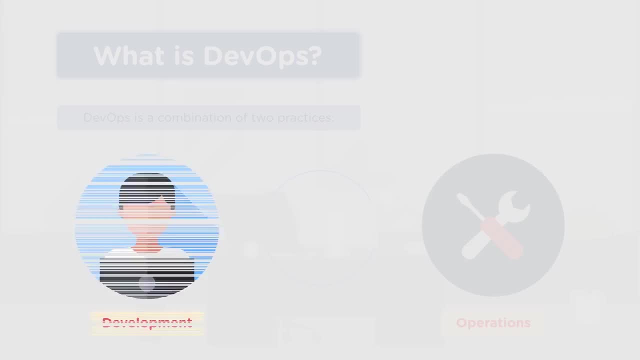 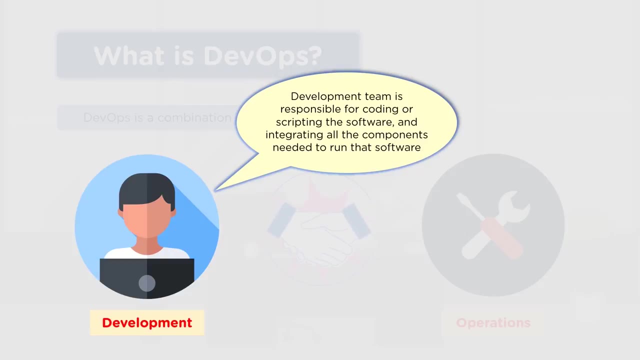 So they take care of all those tasks: creating the virtual machines, managing, performing the patching and number of tasks there from the operations perspective. Now, development is something which keeps on working on the source code there on the development, and they are responsible for keeping a particular product up and running. So they do the performance. they 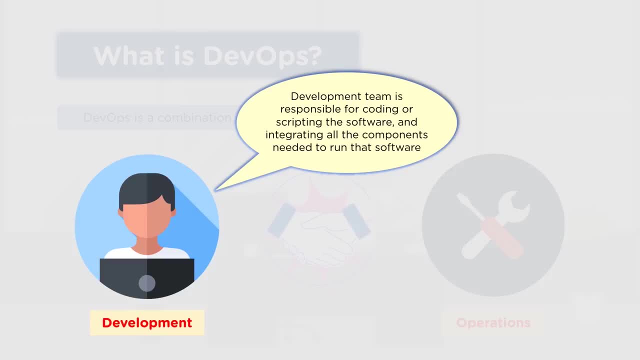 you know they do the coding, they do the particular interaction with the testing to you know, validate their source code. A huge number of activities is actually done by the development team and they eventually uses a number of tools like scripting tools, coding tools, development tools, a lot of tools. 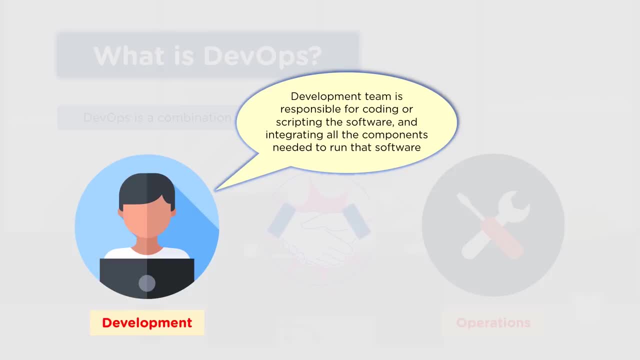 they basically use to support their development. because they are performing different kind of programming, It could be a possibility that more than one programming language is being used for your project, so that's kind of you know. wider scope is present as such over here when we talk about the DevOps here. Now, from the operations, 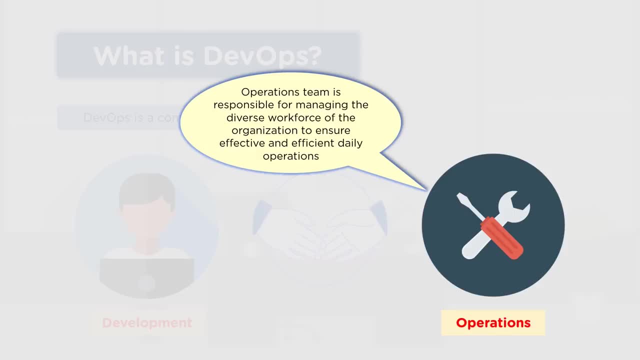 perspective. it's basically a team which is responsible for managing the workforce right and it's something which we can use to see that all the daily activities and operations should be managed effectively and efficient. So that's the main important point over here: that whenever we are working with the 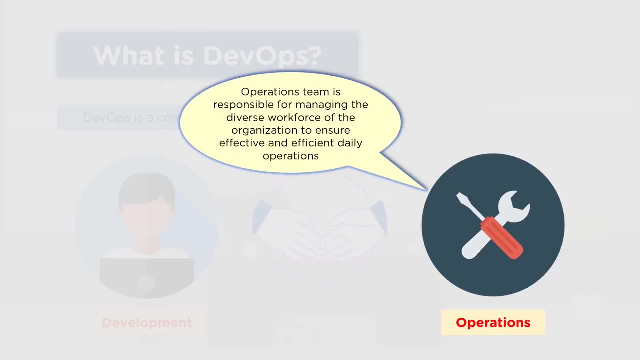 operations. whenever we are working on that, we should be able to get a kind of a decent amount of work and decent amount of activities managed with the help of operations teams here. So operation teams is pretty much responsible for keeping the environment up and running and whatever the 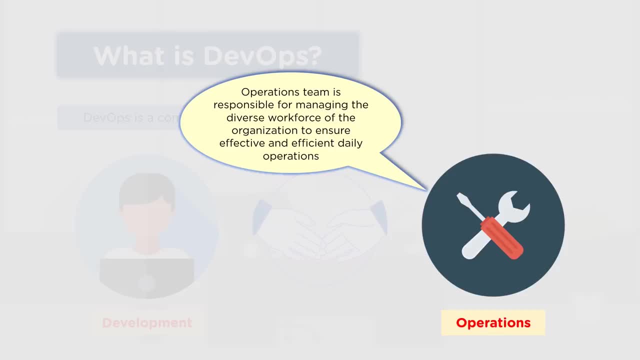 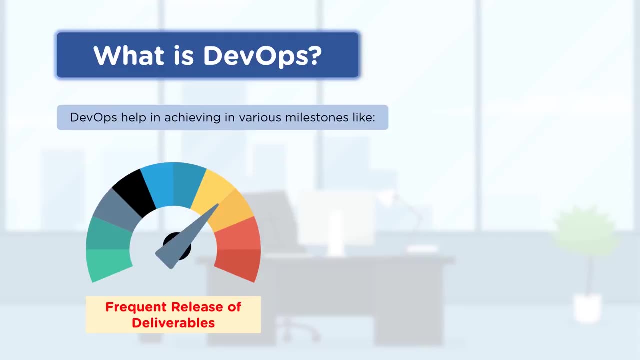 activities and maintenance work we want to do. we will be able to do on that Now. DevOps really helps us to achieve a lot of milestones over here. Now let's talk about that one by one. So very first, one of that is that it helps us to 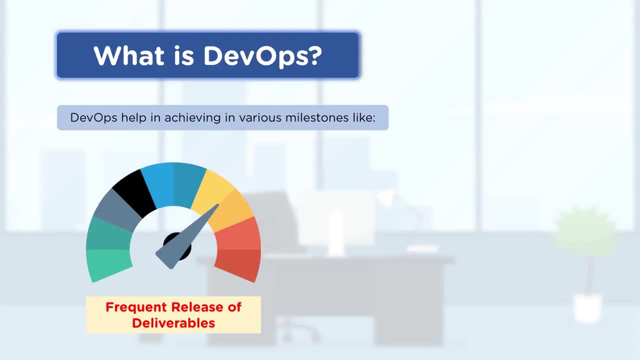 get a frequent release of deliveries here. Now we were doing the releases prior to DevOps also, but that was not that much frequent. Probably people were doing like every quarter, every three months, four months. that kind of time duration was being used by the team to deliver the source code or 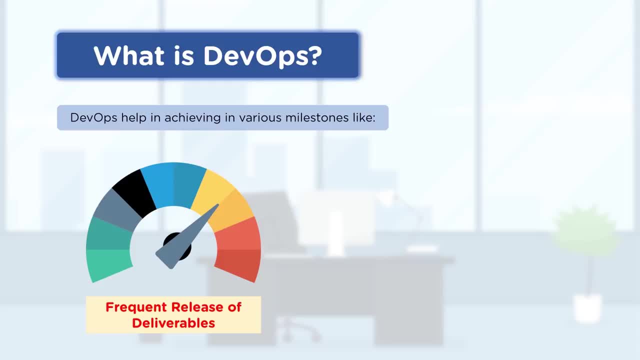 deliver into a specific environment. But the moment the specific DevOps comes into the picture, the frequency of this release really increased a lot. So some organization in fact trying to do like every month, release twice a month. So that's the kind of frequency which we 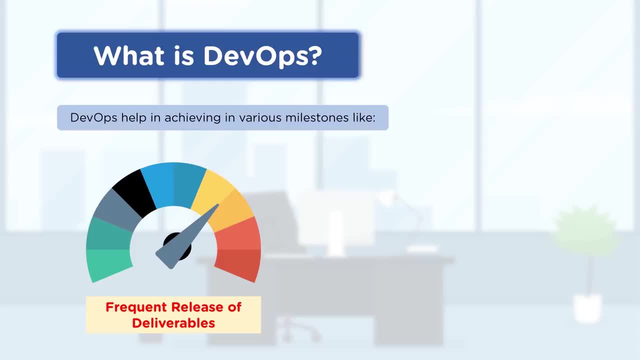 are getting when we move on to the DevOps. So that really helped and, you know, got efficient with the introduction of DevOps here Now. second one is the team collaboration. Now that is also improved drastically because earlier the operations and the development teams were not working in that. 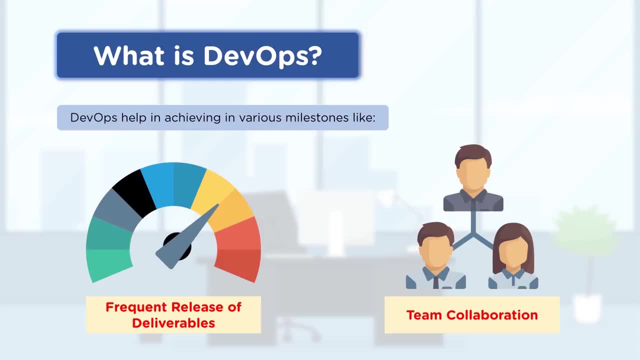 collaboration. They were like working involved in their own tasks, But with the help of DevOps they really come along and, you know, had a very good team collaborations, which really helps them to increase the overall productivity and the performance of the product. So these are the 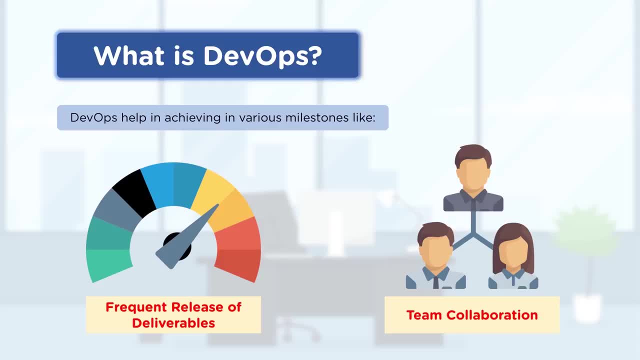 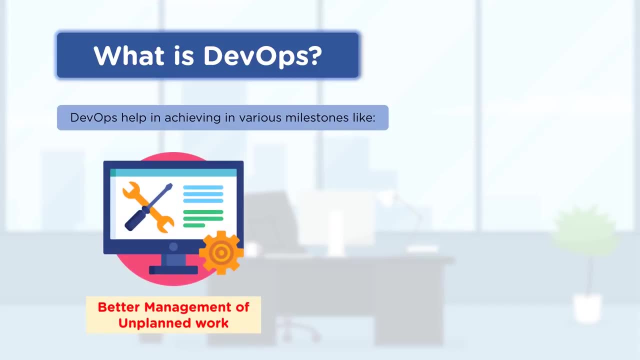 prime milestones which we achieve with the implementation of DevOps as such into our project. Another one is that it helps to get a kind of a management, a better management here. so effective and efficient management is what we get with the help of DevOps, because ultimately, 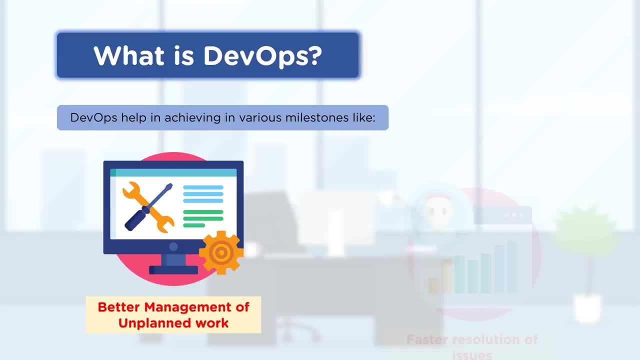 you have redefined your processes, you have implemented certain development tools, certain automations, and that really helps you to increase the overall management of all your unplanned work. So the planning is something which got really improved with the help of DevOps and faster resolution of issues, because the way you are delivering your source code to the production 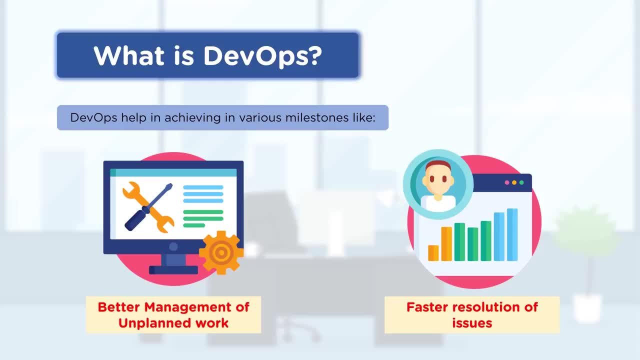 environment. you are pretty much doing it into a less duration of time and when that is happening, definitely there is an kind of a increase in the number of bugs which is getting a result and there is another benefit that you know- ultimately the number of bugs which you are getting in production- that drastically reduced. 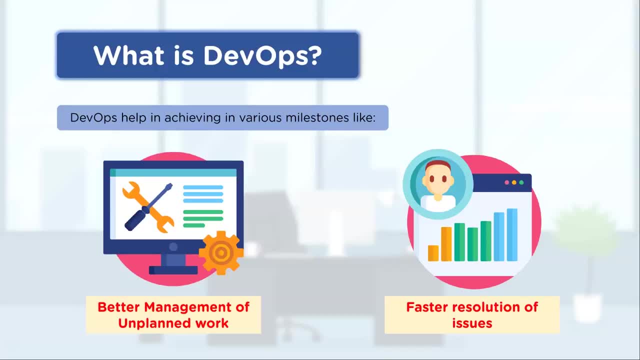 in case of DevOps. So since we are getting less number of issues and bugs, it's very easy for us to do the resolutions quite quickly and implement into a specific production environment, Right? so DevOps today is being implemented by, you know, most of the major organizations. 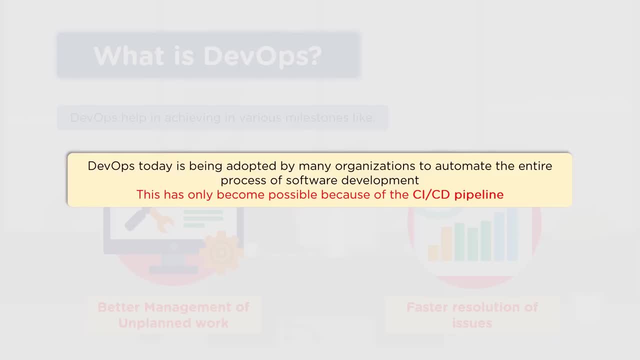 whether it's a financial organization, whether it's a kind of a service organization, every organization is somehow looking forward for the implementation and the adaptation of DevOps, because it totally redefines and automate the whole development process all together and, whatever the manner efforts you were putting earlier, that is simply or gets automated with the help of these tools here. 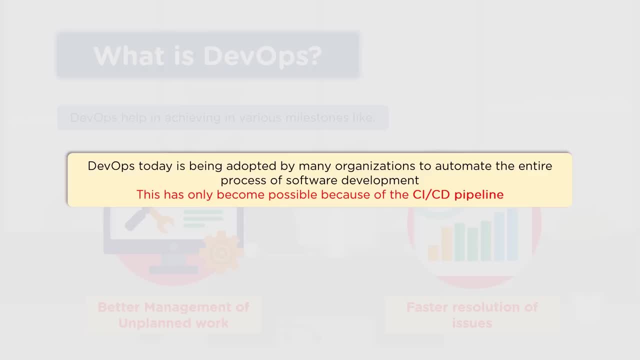 So this is something which get really implemented because of some of the important feature like a CI CD pipeline, because CI CD pipeline Is responsible for delivering your source code into the production environment in less duration of time. So CI CD pipeline is ultimately the goal which really helps us to deliver. 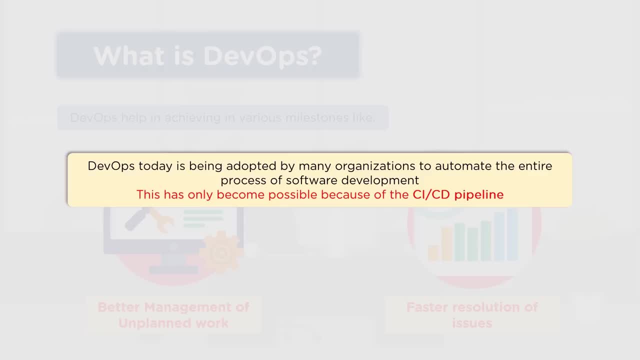 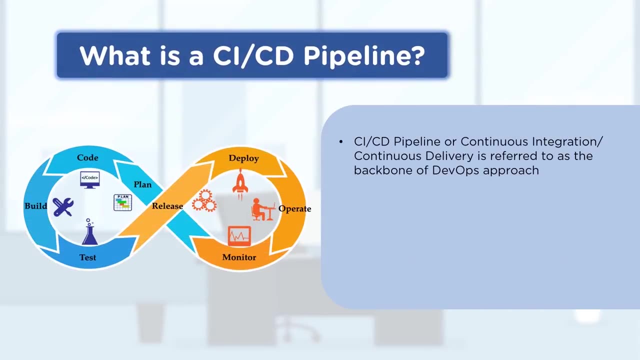 more into the production environment when we talk about from this perspective, Now, let's talk about that. what exactly is a CI CD pipeline? Now, when we go into that part, when we go into that understanding, so CI CD pipeline is basically continuous integration and continuous delivery concept which is used or which is considered as an backbone of the 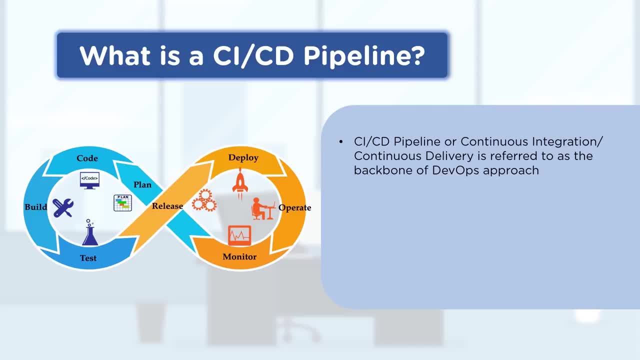 overall DevOps approach. Now it's one of the prime approach which we implement when we are going for a DevOps implementation for our project. So if I have to go for a DevOps implementations, the very first and the minimum implementation and the automation which I'm looking forward is actually 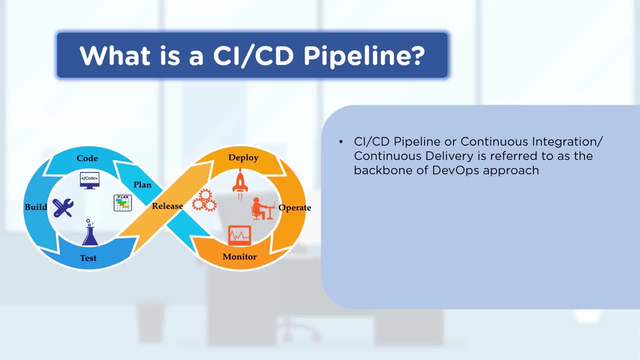 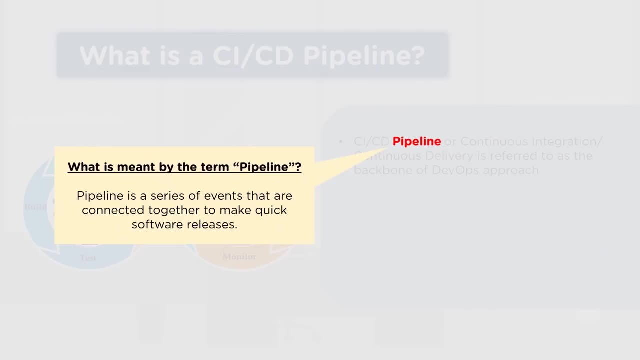 from the particular CI CD pipelines here. So CI CD pipelines is really a wonderful option when we talk about the DevOps here. So what exactly is the pipeline term all about? So pipeline is a series of events that are connected together with each other. It's kind of a. 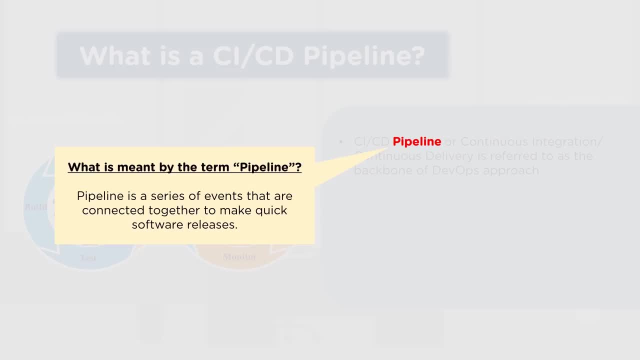 sequence of the various steps. like you know, typically when we talk about any kind of deployment, So we have, like you know, built process like we compile the source code, which, under the artifacts, we do the testing and then we deploy to a specific environment All these various 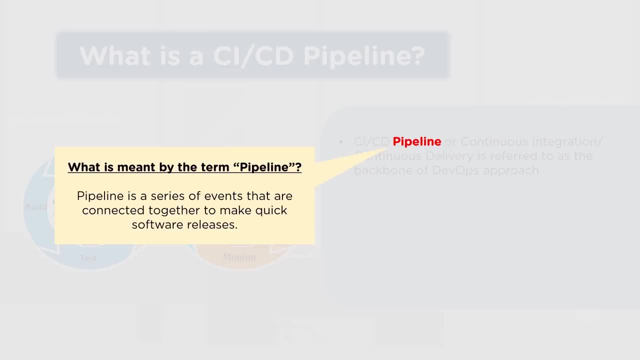 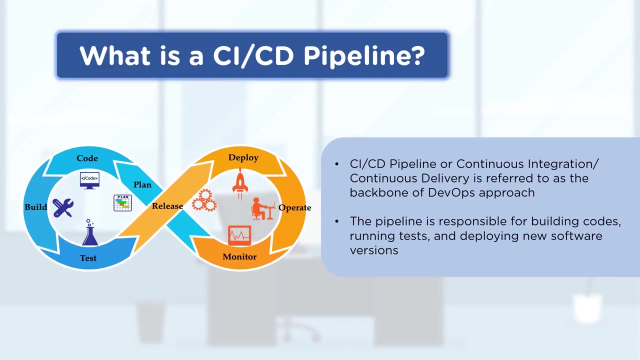 steps which we used to do it like manually. That is something which we can do it into a pipeline. So pipeline is nothing but a sequence of all these steps interconnected with each other, Executed one by one into a particular CI CD pipeline sequence. Now the pipelines is responsible for performing a variety of tasks like building up. 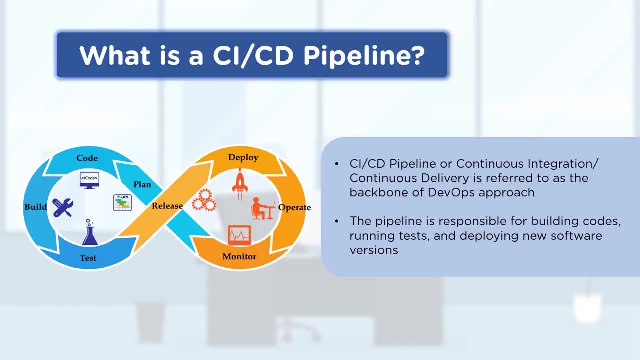 the source code running the test cases. probably the deployment can also be added up in when we go for the continuous integration and continuous delivery there. So all these steps are being done into a sequence, definitely because sequence is very important when we talk about the pipeline. 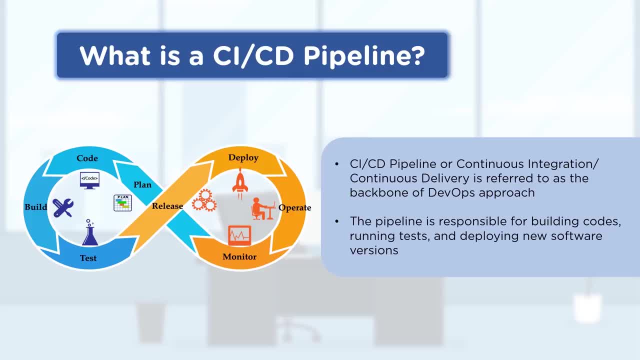 So you need to talk about the sequence: the same way in which you are working on the development and, in a typical world, the same thing you will be putting up into a specific pipeline. So that's a very important aspect to be considered. Now let's talk about what is the Continuous Integration here. 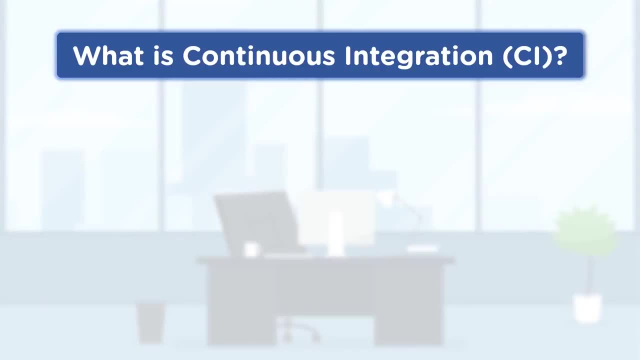 Now continuous integration is also known as the CI. pretty much you can see that lot of tools are actually named as CI, but they are referring to the Continuous Integration only. So continuous integration is a practice that integrates the source code into a shared repository and 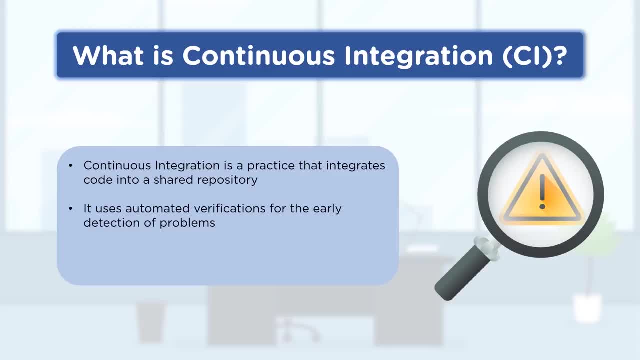 a. it used to automate the verification of the source code, so it involves the build automations, test cases automation, so it also helps us to detect the issues and the bugs quite easily and quite faster. that's a very early mechanism which we can do as such if we want to resolve. 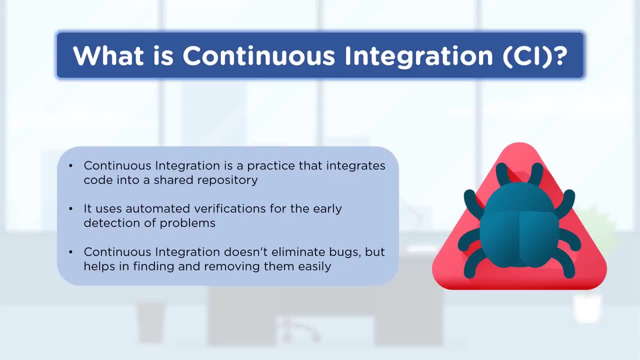 all these problems. now, continuous integrations does not eliminate the bugs, but yes, it definitely helps them. uh, you know easily to find out because we we are talking about the uh automated process, we are talking about the automated test cases. so definitely that is something which can help us to. 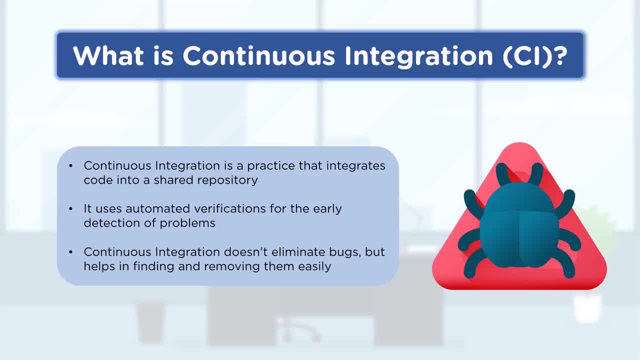 uh, find out the bugs and then you know the development can help on that and they can, you know, proceed with those bugs and they can try to resolve those things one by one. so it's not a kind of automated process which will eventually remove the bugs. bugs is something. 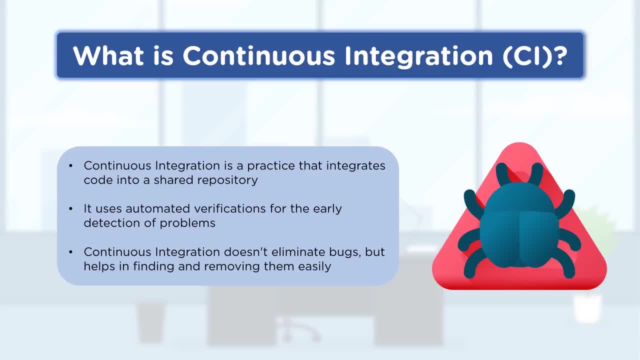 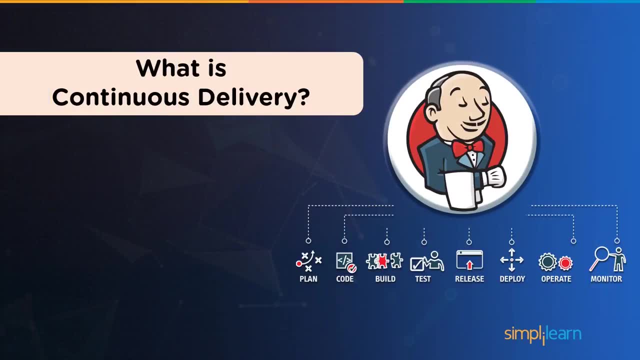 which you have to record and you have to fix it by following the development practice. but yes, it can really help us to find those bugs quite easy and help them to remove. now, what is continuous delivery here? so continuous delivery, also known as cd, is in kind of a phase in which 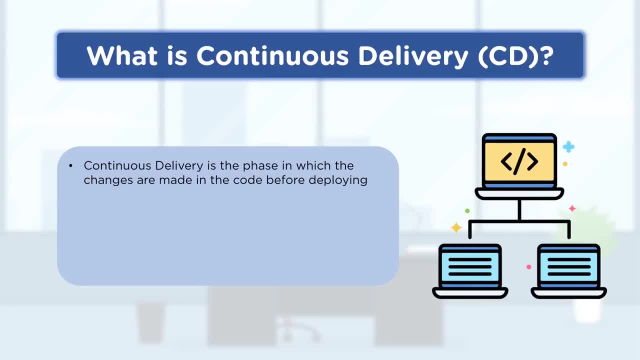 the changes are made, uh, into the code before the deployment. now, in this case, what happens that? uh, it's, um, something which we are discussing, or we are validating that. what exactly we want to deliver it to the customer. so, what exactly? we are going ahead or we are moving to the 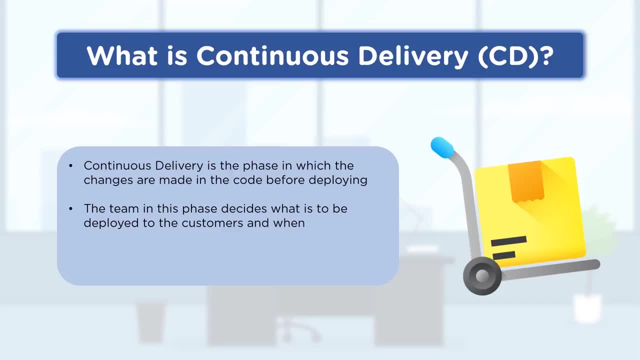 customer. so that's what we typically do in case of continuous delivery, and the ultimate goal of the pipeline is to make the deployments. that's the end result, because coding is not the only thing. you code the programs, you do the development. after that it's all about the 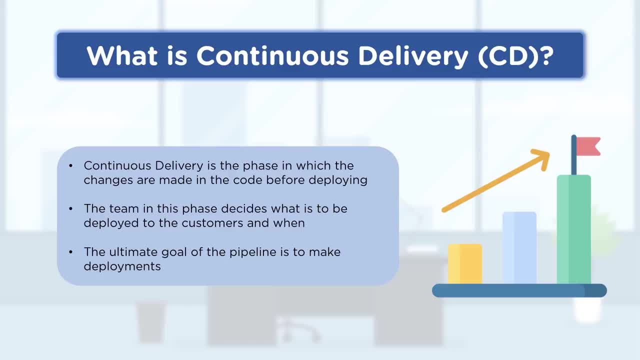 deployments, like how you're going to that to perform the deployment. so that is a very important aspect. you want to go ahead with the deployments, that's right, you can go there. and that's the real beauty about this, because it it's in kind of a way in which we can identify. 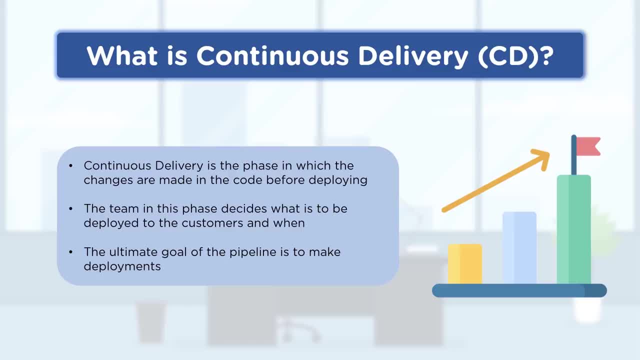 that how the deployments can be done or can be executed as such here. right? so the ultimate goal for the pipeline is nothing but to do the deployments and to proceed further on that, right so when both these practices are placed in together in an order, so all the steps could 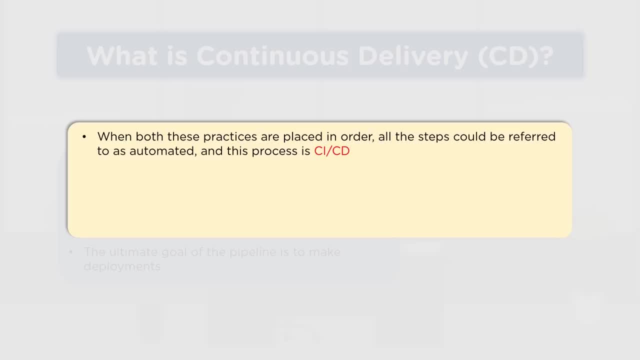 be referred as in complete automated process, and this process is known as cicd. so when we are talking about, like when we are working on this automation, so in that case what happens? that we are looking forward, that how the automation needs to be done, and since it's in kind of a cicd, 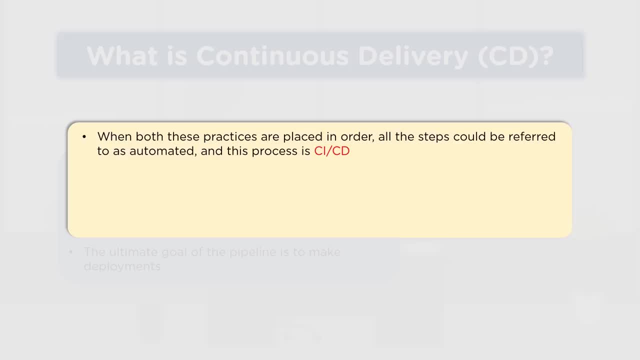 automation which we are talking about. so it's nothing but the uh end result would be like build and deployment automation. so you will be taking care of both the build and the test case executions and the deployments as such when we talk about, as such, the cicd here. the implementation of cicd also enables the team. 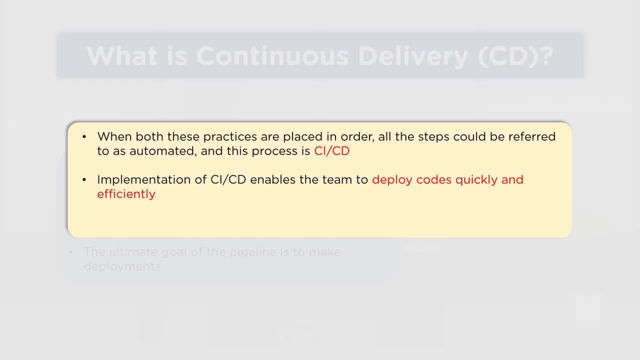 to do the build and deploys quite quickly and, uh, efficiently, because these are things which is, you know, happening automatically, so there is no manual efforts involved and there is no scope of human error also. so we have frequently seen that while doing the deployments, we may miss some. 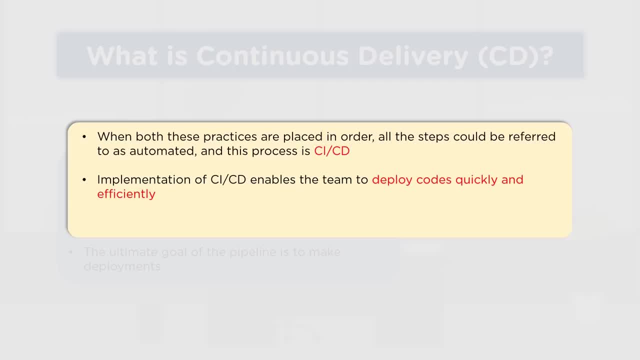 boundaries or some miss can be there. so that is something which is, you know, completely removed as such when we talk about this. the process makes the teams more agile, productive and the uh confident here because, um, the automations definitely gives a kind of a boost to the. 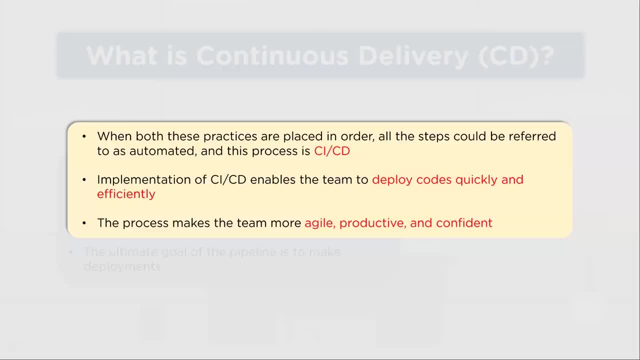 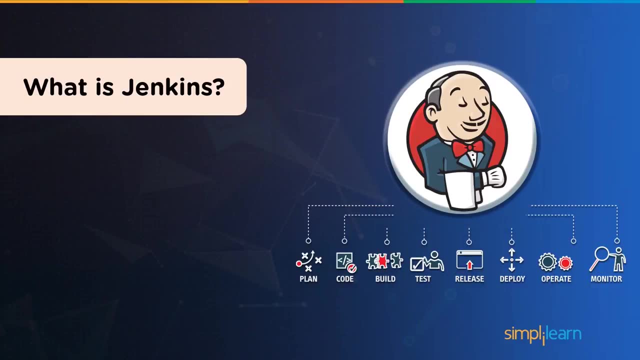 confidence that, yes, things are going to work perfectly fine and there is no issues as such present. now why exactly jenkins? like jenkins is what we typically understand, or we you know, uh, here and there that it's in ci2, it's a cd tool. so what exactly is jenkins all about? so 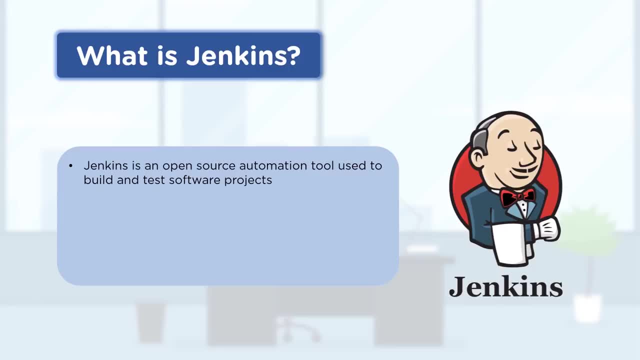 jenkins is also known as a kind of orchestration tool. it's an automated tool which is there and the best part is that it's completely open source. yes, there are some particular uh paid or the enterprise tools are there, like cloud, bs and all, but there is no as such. 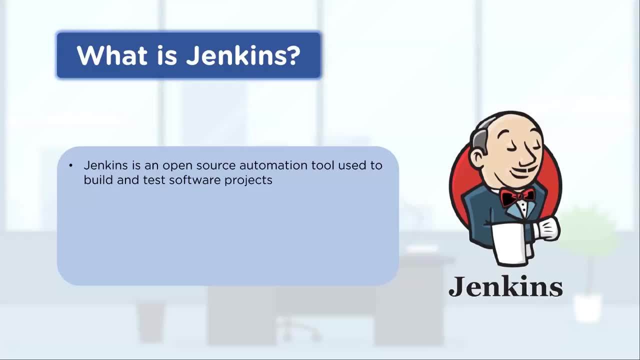 of offering difference between the cloud bs and the jenkins here. so jenkins isn't kind of open source tool which a lot of organizations pretty much implement as it itself. so even if they don't want to go um, we have seen in a lot of big organizations where you know they are not going for the enterprise. 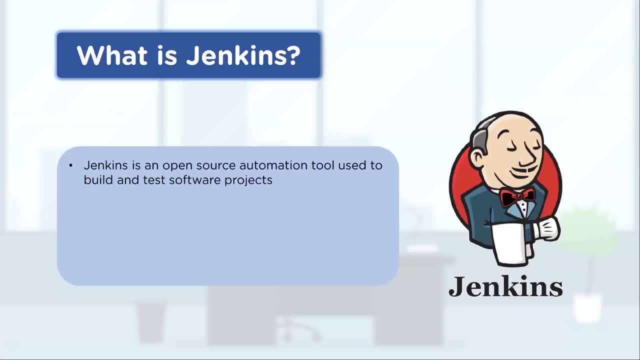 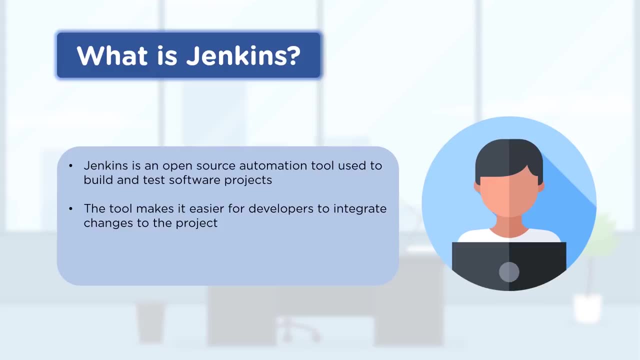 tool like cloud bs and all, and they are going for the pretty much you know core jenkins software as well. so this tool, uh, makes it easy for the developers to integrate the changes to the project. that is something which is very important because it can really help the teams to say that. 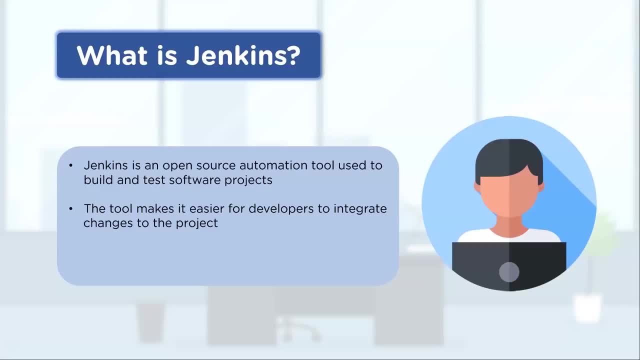 how the things can be done and how it can be performed over there. so the tools is really easy for the developers to integrate and that's the biggest- uh, you know- benefit which we are getting when we talk about these tools as such. so jenkins is a really important tool to be. 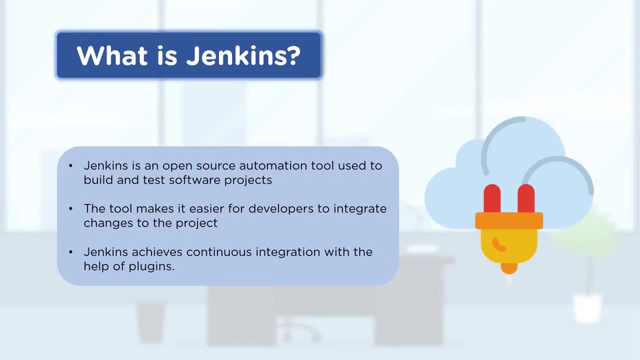 considered when we talk about all these automations. now, jenkins achieves continuous integration with jenkins. that is also a kind of another feature or benefit which we get, because there are so many plugins which is available there as such, which is being used and uh, for example, you want to have an. 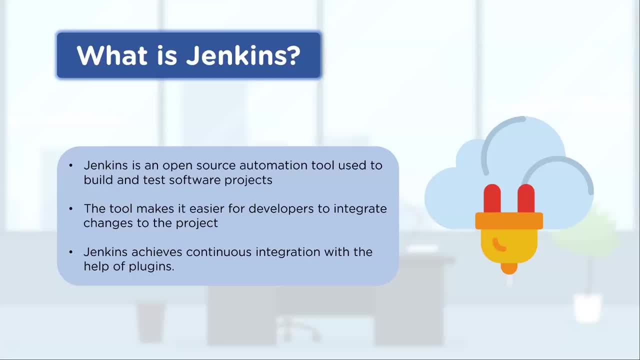 integration with kubernetes, docker and all. maybe by default those plugins are not installed, but yes, you have the provisioning that you can go for the installation of those plugins and, yes, those features will start embedded up and integrated within your jenkins. so this is the reason, this is the main benefit which we get when we talk about the jenkins implementation. 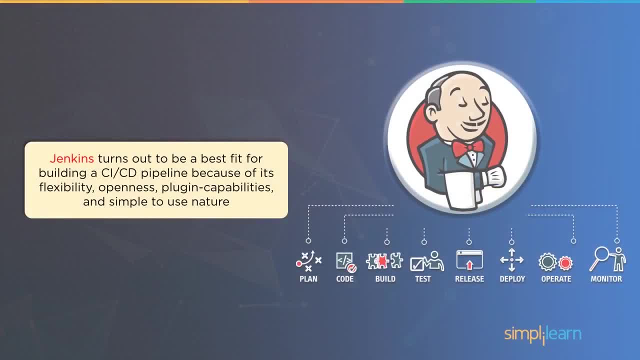 so, jenkins, uh, is you know one of the best fit which is there for building a cicd pipeline because of its flexibility? uh, open source, nature, plug-in capabilities, the support for plugins, and it's quite easy to use and it's very simple, straightforward gui. which is there which can? 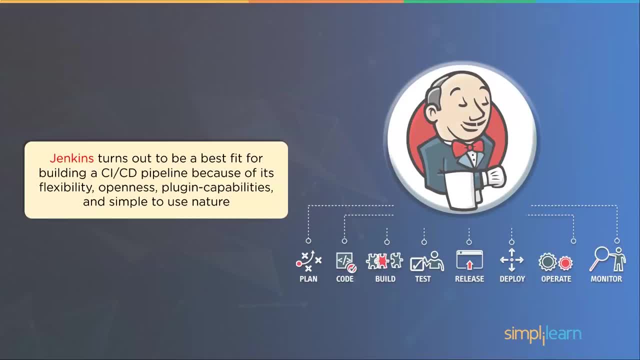 definitely helps us. you can you know, easily understand and go through the jenkins and you can grab the understanding and, as an end result, you will be able to have a very robust tool which, using which pretty much any kind of source code or any kind of programming language, you can implement cicd, whether it's an android, it's a. 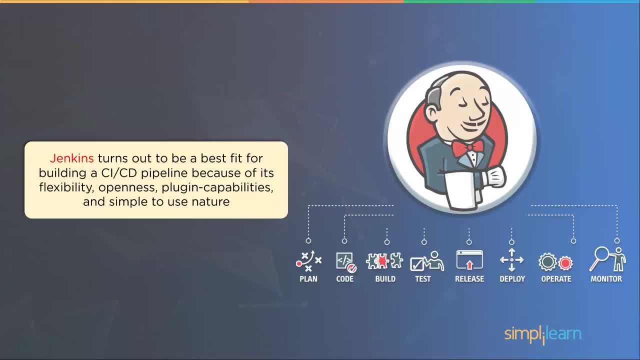 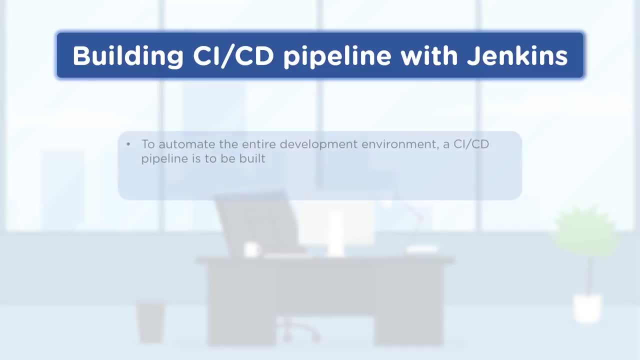 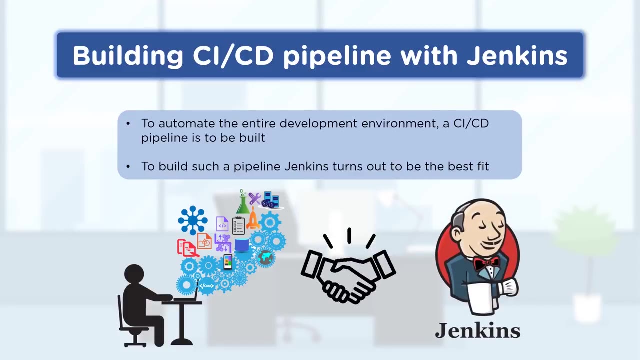 nordnet. it's a java, it's a nodejs. all the languages are having the support for the jenkins. so let's talk about the cicd pipeline, with the jenkins here now to automate the entire development process. a cicd pipeline is the ultimate you know solution which we are looking forward to build. 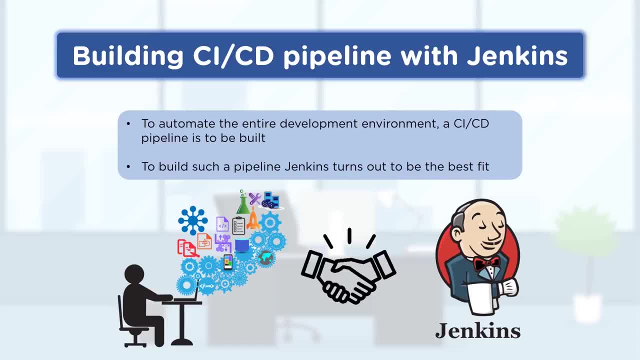 such a pipeline, jenkins is our best solution and best fit which is available here. so there are pretty much six uh steps to build a jenkins pipeline. first of all, the first step is to build a jenkins pipeline, which is a basic pipeline, which is a generic pipeline, in order to build a jenkins- jenkins. 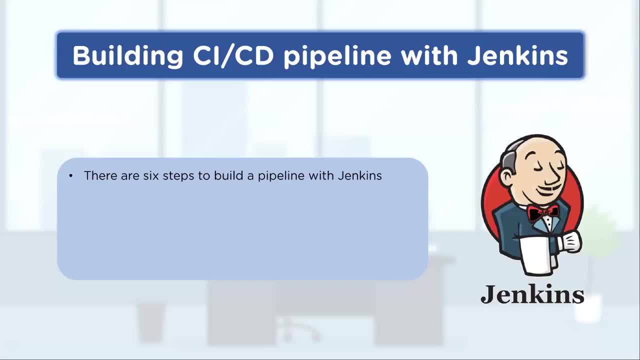 pipeline, which is a generic pipeline which we are looking forward to. now it may have, like, uh, another steps which is available there, probably some additional steps you're doing, like some other plugins you are installing, but these are the basic steps which is there, like a minimum pipeline if you want to design. these are the steps which is available there. now let's see. 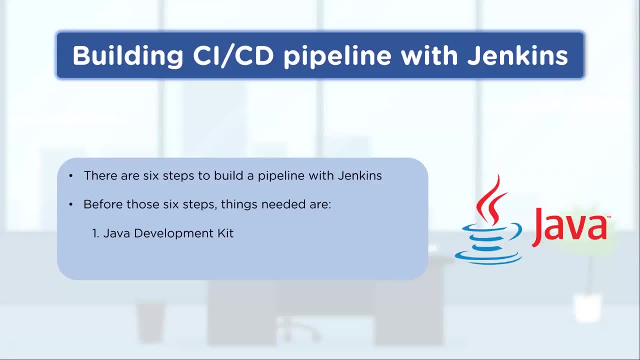 the first one is that we have the uh required java jdk, like uh jdk, to be available on the system. now most of the operating systems are already available with a gre Java GRE, but the problem with GRE is that it's only for the build process. It will not be doing. 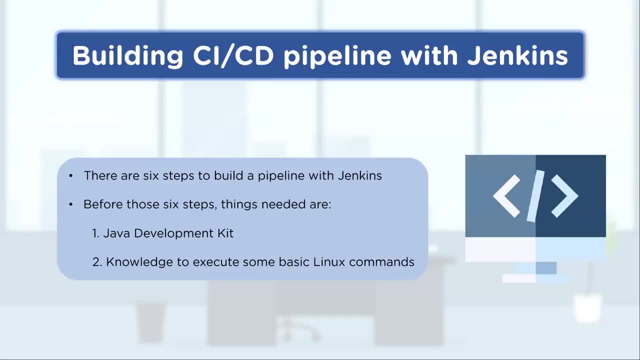 the compilation. You can run the artifacts, you can run the jar files, you can, you know, run the application, run the code base. but the compilation requires the Java C or the Java JDK kit to be installed onto the system, and that's the reason why, for this one, we also require the JDK and 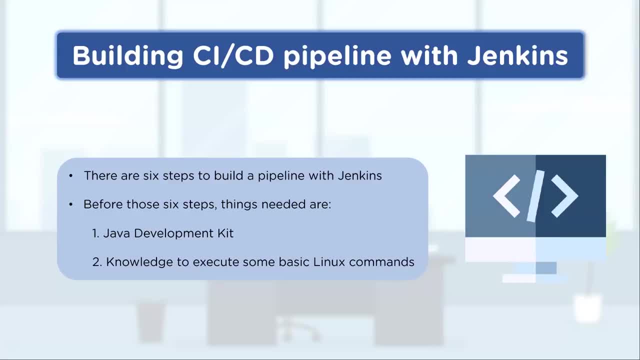 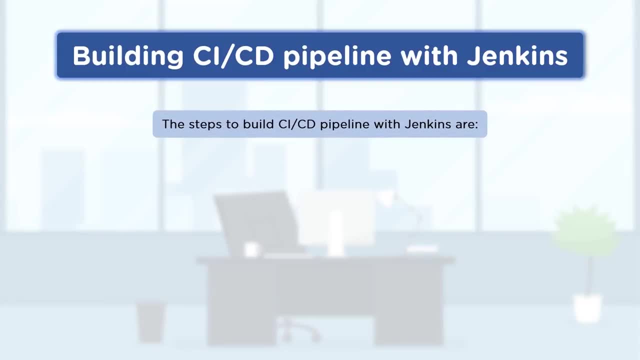 certain Linux commands execution understanding we need to have because we are going to run some kind of steps, some installation steps, and you know process, so that's pretty much required. Now let's talk about how do CACD pipeline with Jenkins. Now, first of all you have to download the JDK. 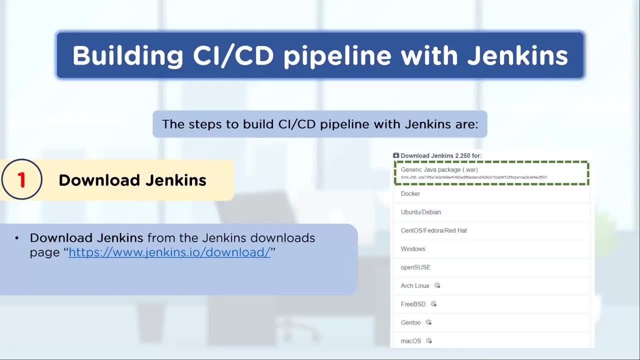 and that is something which is installed, so after that you can go for the Jenkins download. Now jenkinsio slash download is the website. is the official websites of Jenkins. Now, the best part is that there you have support for different operating systems and platforms. From there you 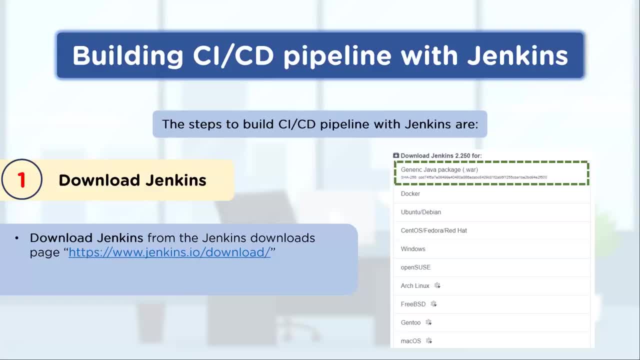 can easily say that if you want to go for a Java package like a war file talker, ubuntu, dev file, you can easily say that if you want to go for a java package like a war file talker, ubuntu, devian, CentOS, ferora, redhat, windows, opensuche, freebsd, ganto, mac operating system. 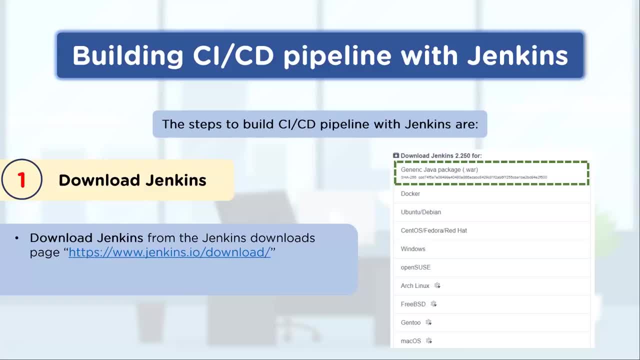 In fact, whatever the different kind of artifacts or different environment or different application you want to download, you will be able to do that. So that's the very first thing to start upon. You download the generic java package like a war file. then you have to execute. 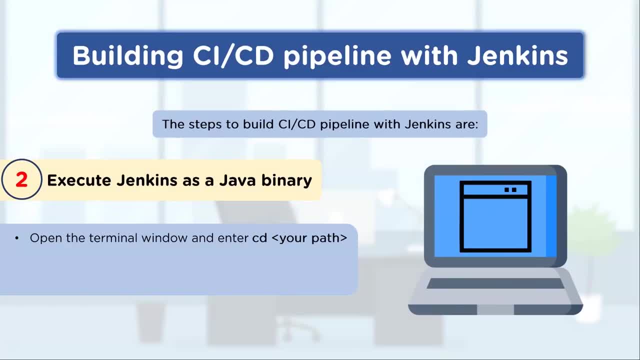 it. You have to download that into a specific folder structure. Let's say that you have, you know, created a folder called jenkins. Now you have to go into that jenkins folder with the help of cd command and there you have to run the command called java hyphen jar. 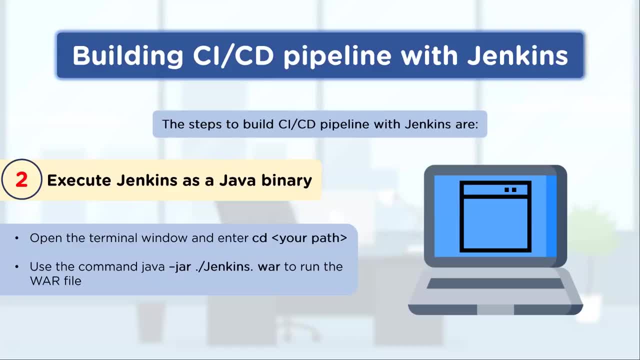 and the jenkinsvar there. So these are the executables artifacts. So war files can be easily executable. Jar files, war files, can be easily deployed. So just because with the java command you can run them, you don't require any kind of web container or application container. 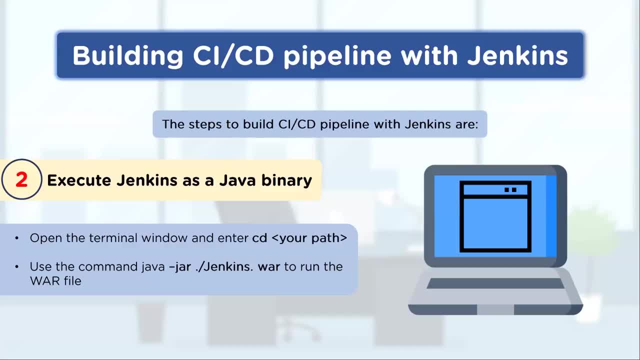 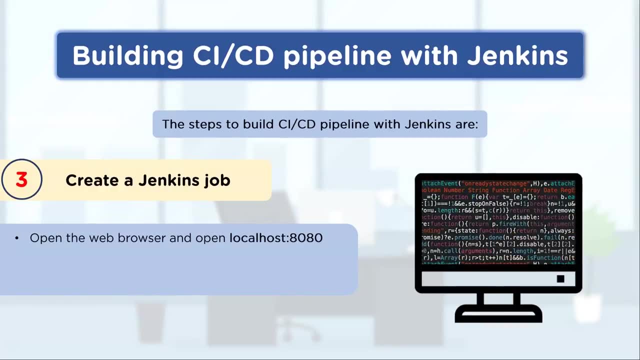 as such. So here also you can see that we are running the java command and it runs the applications as such And once that is done so you can open the web browser and you can open like localhost, colon 880.. So jenkins uses the 880 port just. 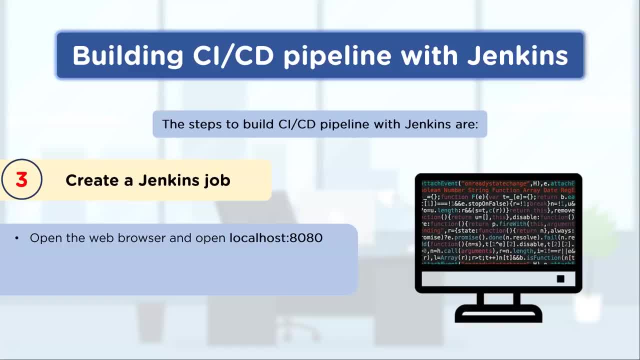 like a tomcat apache. So, if you know, once the deployment is done, installation is done, so you can just open the localhost colon 880.. Now if you want to get the jenkins up and running in the browser, probably you can, you know, go through the public ip address also there So you can put. 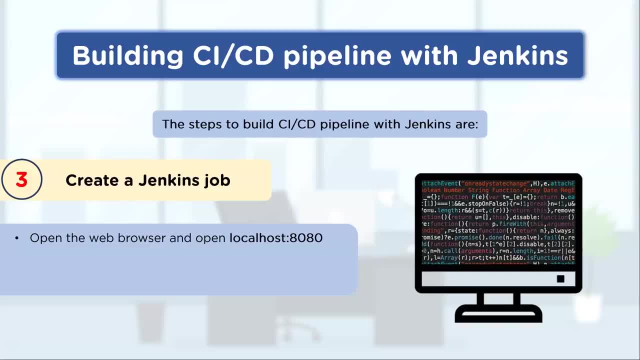 the public ip address, colon 880, and that can also help you to. you know, start accessing the jenkins application Now. in there you will be having an option called create new jobs. So you need to click on that Now once the particular new job, new item, new job- that's a different naming conventions which is 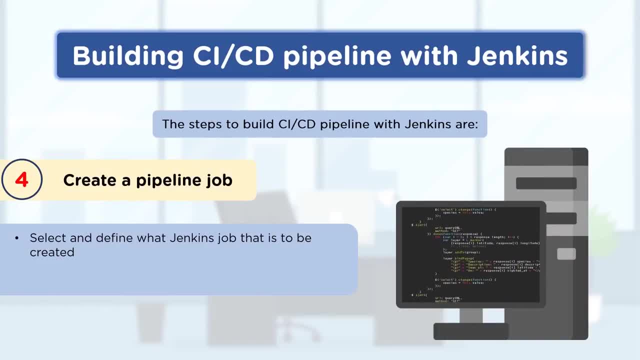 available there. Now all you are going to do is that you're going to do like you are proceeding with the creating the pipeline job, So you will be having an option called pipeline job over there. Just select that and provide your custom name. what pipeline name or job name you want to refer. 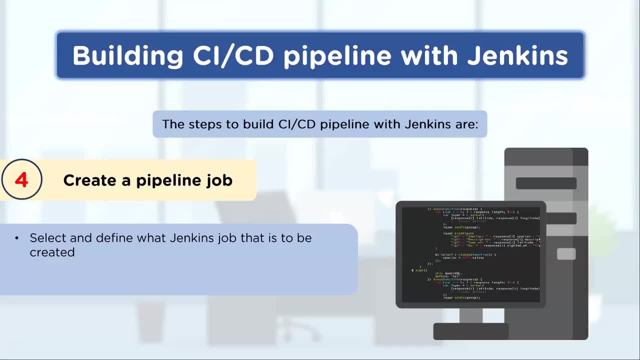 or you want to process there Now, once that is available. so what happens? that it will be in easy task for us to see that how exactly we can go ahead and we can perform on that part. So this can really help us to see that how a pipeline job can be created and 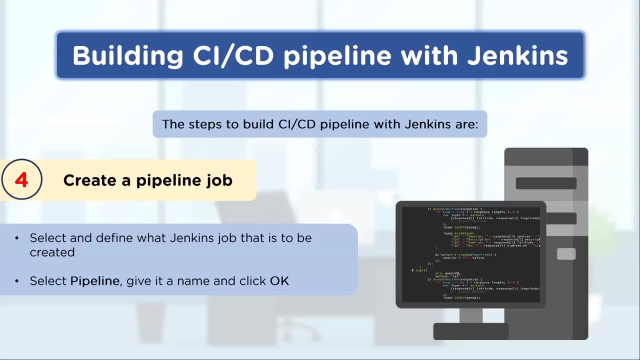 you know, performed on these modifications as such. Now, when the pipeline is selected and we can give a particular name, that this is the name which is available, and then we can say, okay, as such. over there Now you can scroll down and find the pipeline section. So there, what happens? that when you go over there and say that, okay, this is the way that how the pipelines are doing over here. 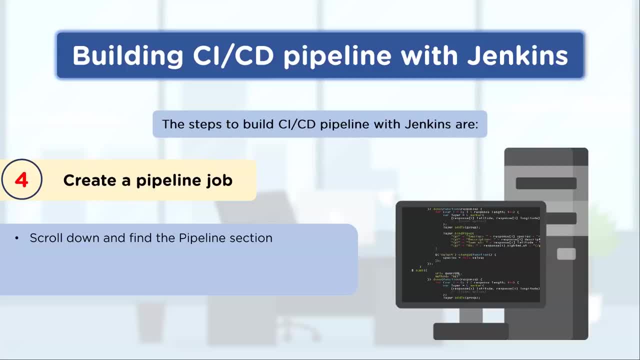 are managed and you know those kind of things. so you will scroll down and find the pipeline section and go with that pipeline script. now, when you select that option, there are different options which is available, like how you want to manage these pipelines. now you are, you know, have the 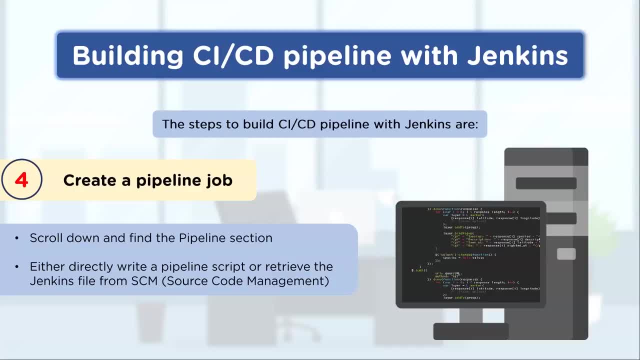 direct access also, like if you want to directly create the uh, create a pipeline script, you can do that. if you feel that you want to manage like you want to retrieve the jenkins files also, scored management tool also can be used there, so you can work on that also. so like this: there are so many a. 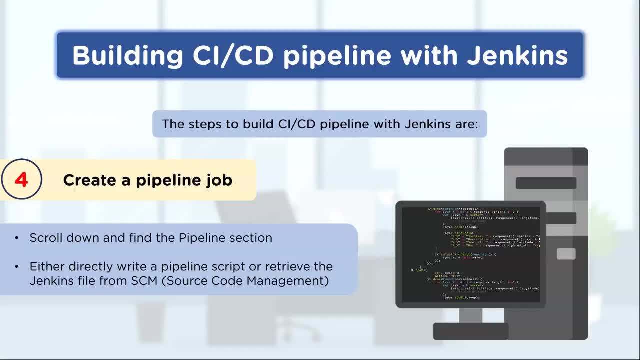 variety of things which is available, like which you can use to work around that, how exactly the pipeline job can be created. so either you can fetch it from the source code management tool, uh, like git subversion or something like that, or you can directly put the pipeline code as such. 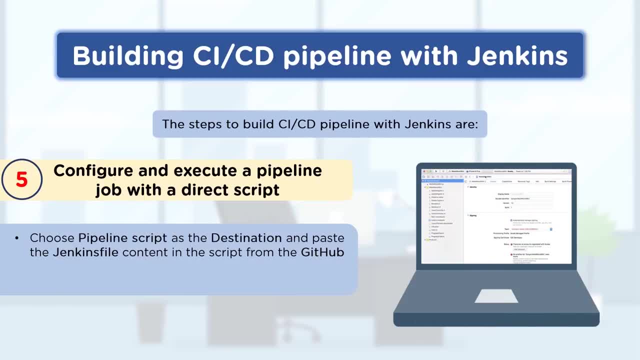 over there right now. so next thing is that we can configure and execute a pipeline job with the direct script. so, uh, we can. once the pipeline is selected, so you can put the uh script, like jenkins file, into your uh particular github link. so you- you may be having like already- 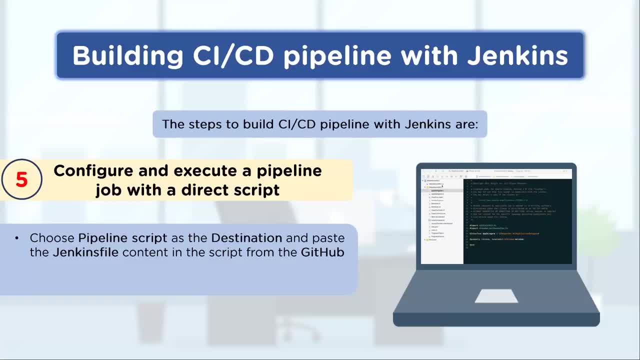 a github link so that the where the jenkins file is there, so you can make use of that now, once you process the github link. so what we can do is that we can proceed with that and, uh, once the processing is done, so you can do the save and you know you can keep the changes and 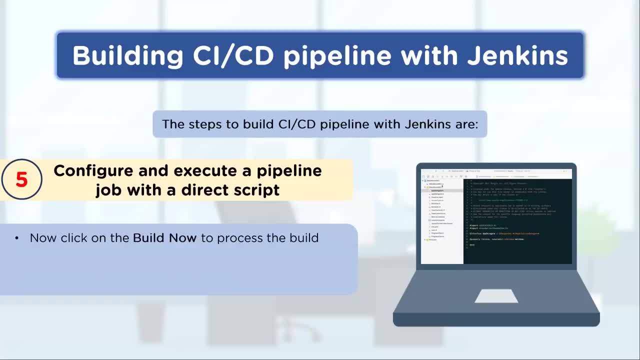 you know, uh, it will be picking up the pipelines. you know the pipeline script is added up into the uh github and you know you have already specified that. uh, let's just go ahead with this jenkins file pipeline script from the github repository and proceed further now, once that is done. so what next you can do is that you can go with the build now. 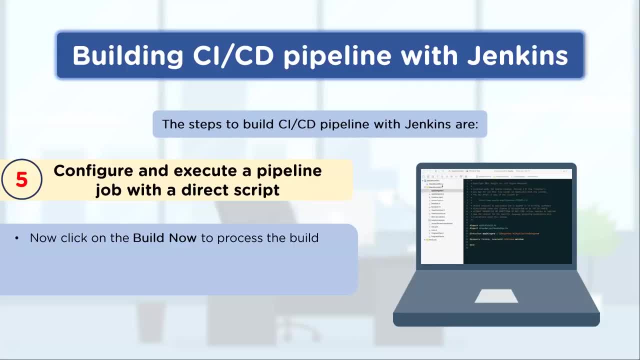 process. you click on the bill now and once that is done, so what will happen? that you will be able to see that, how the build process will be done and how the build will be performed over there. so these are pretty much a kind of a way so you can click on the console output. you will get all the logs. 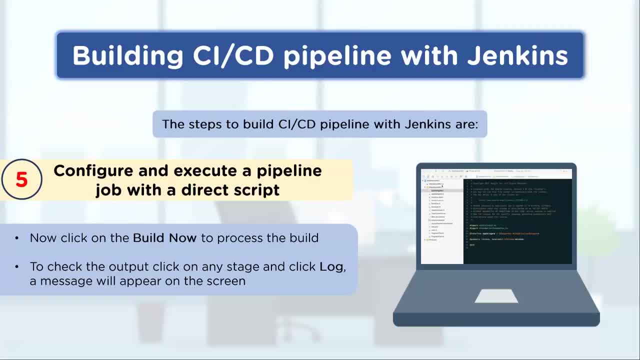 that is happening in the inside, that whatever the pipeline steps are getting executed, all of them you will be able to get, or you will be able to, you know, get on that part there. so these are the different steps which is involved as such, and uh, the sixth one is that you know, uh, yes, whatever the 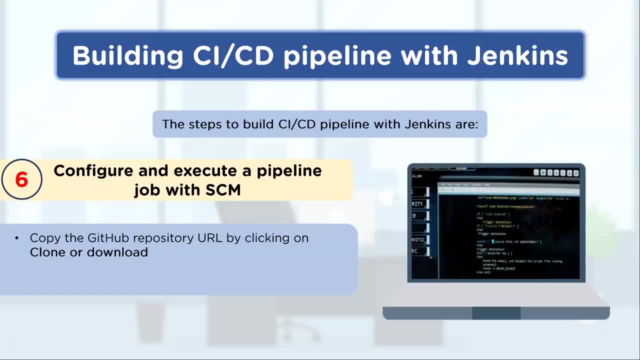 uh, particular uh. when you run the build now, you will be able to see that source code will be- uh, you know, will be checked out and will be downloaded before the build, and you can proceed with that part now. later on, if you want to change the url of this github, you can configure the job again. 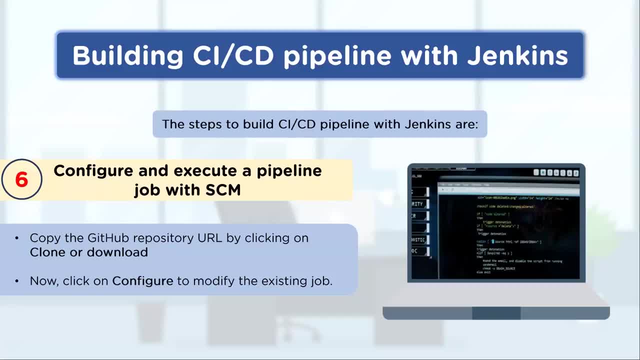 the existing job and you can change that url, github link url whenever you require. you can also clone this uh job whenever you go ahead and you work on that and that's also kind of you know, the best part which is available as such right and uh, then you can have the advanced settings. 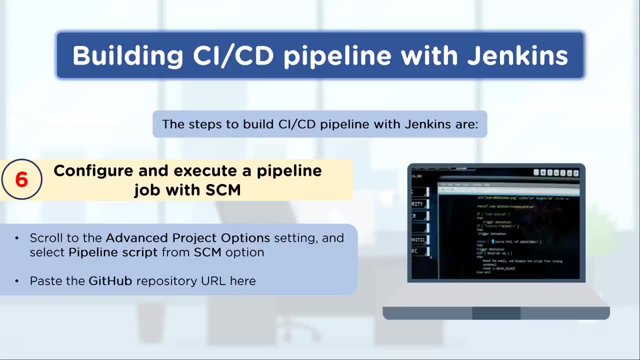 over there, so in there you can put like your github repository. you can say like: okay, uh, the github repository is there, so i'm just going to put this url and you know with that what will happen: that the settings will be available there and the jenkins file. 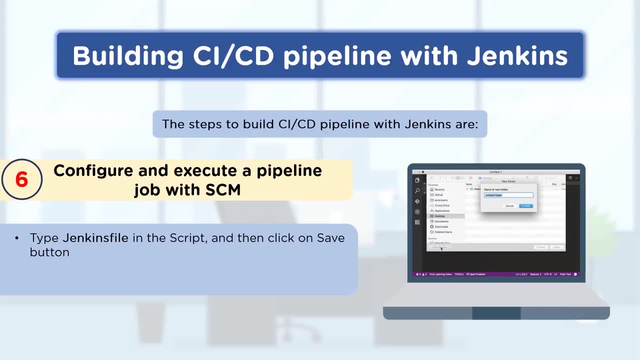 will be downloaded as such and when you run the build now, you will be able to have a lot of steps, like a lot of configurations going on. so, uh, then the checkout scm, so we can have a declaration like checkout scm, which is there. so when the checkout scm is there, so it will check out a specific source. 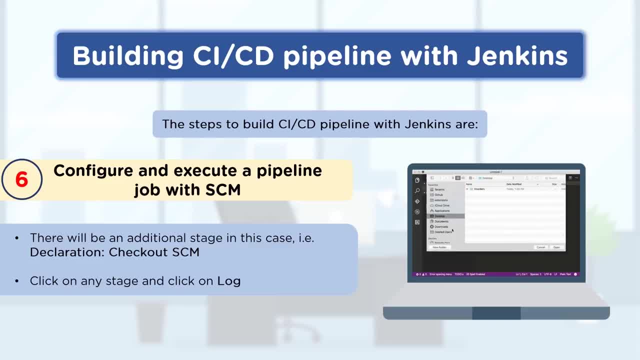 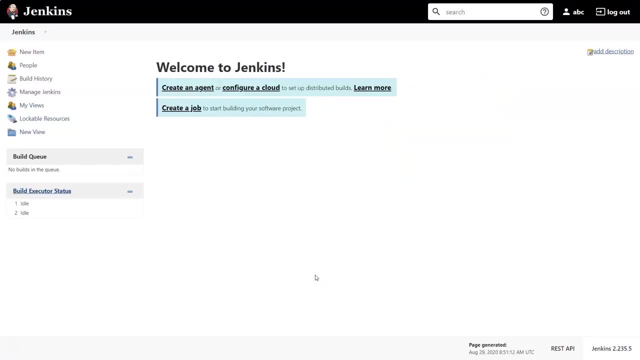 code. after that, you go to the log and you will be able to see that each and every stage which is being built up and executed as such. okay, so now we are going to talk about a demo here. so, uh, the pipeline here. so this is a jenkins portal. now you can see here that there is an option called 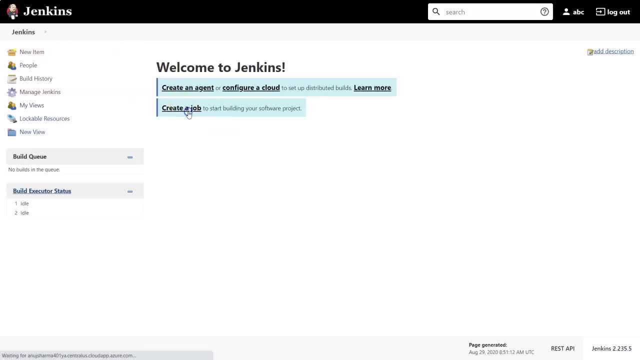 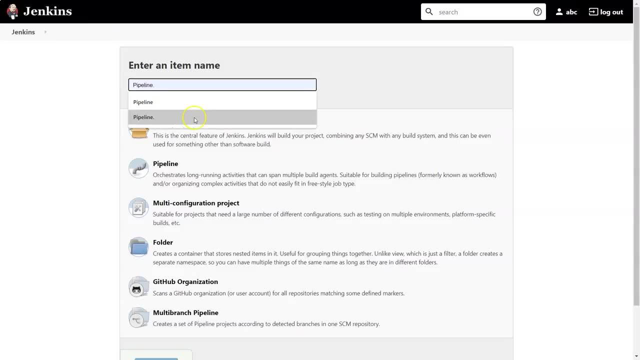 create a job. you can either click on the new item or you can click on the new uh, create a job here now. here i'm going to say like a pipeline and uh. then you know you can select the pipeline, uh job type here. now you have the freestyle pipeline, github organization multi, multi branch pipeline. 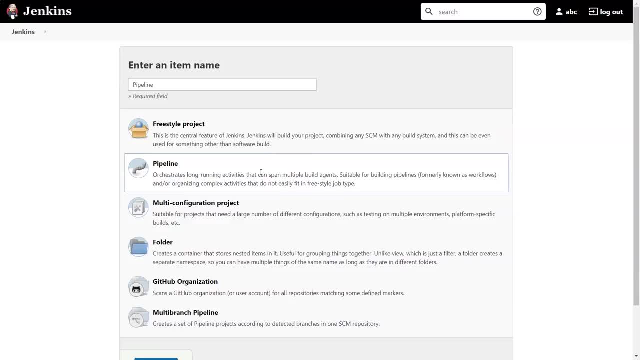 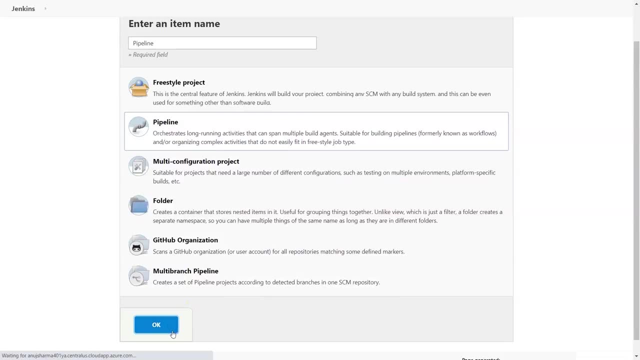 these are the different options which is available there, but i'm going to continue with the pipeline here as such. so when i select the pipeline, i'm going to select the pipeline here as such. so when i select the pipeline and say, okay, so what will happen? that i will be able to see a configuration. 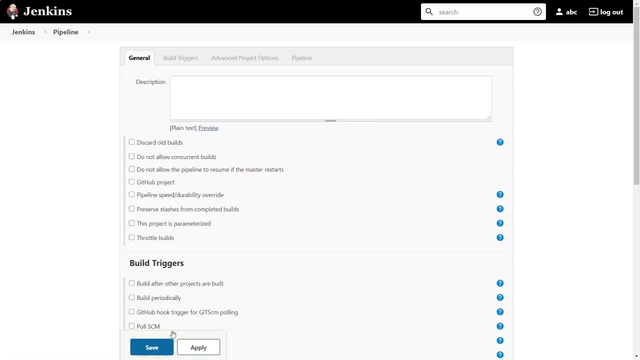 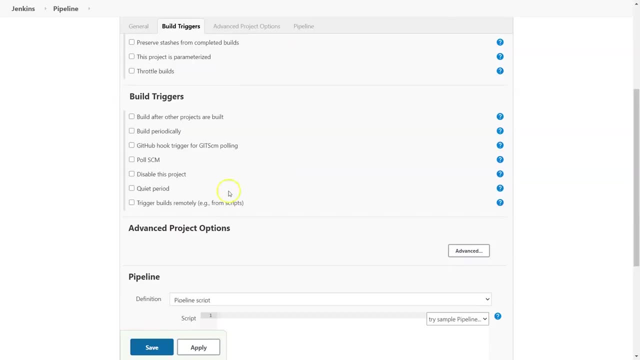 page which is related to the pipeline. now, here, the very important part is that you have all the uh general build trigger, uh, you know options, which is similar to the freestyle, but the build step and the post build step is completely removed because of the pipeline introduction. now, here you either. 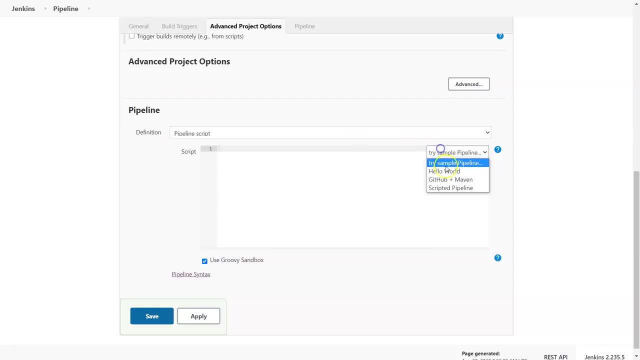 have the option to put the pipeline script all together. you can also have some particular example. for example, let's talk about some github, maven, uh particular uh tool here, so you can see that, uh, we have, you know, got some steps as such over here and you know it's pretty much running over there. now you run it, it will work smoothly, it will check. 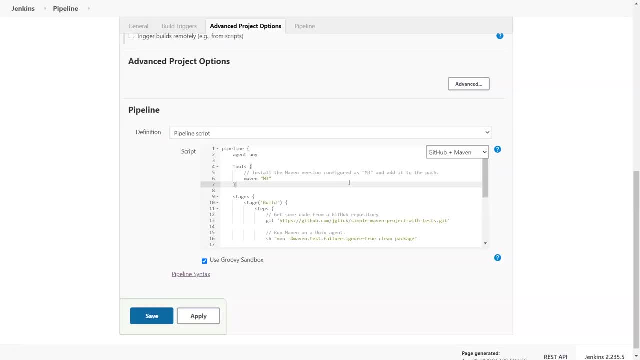 out some source code, but how we are going to integrate, like the version, the jenkins file into the version control system, because that's the ideal approach we should be following when we create a pipeline of a cicd. now i'm going to select a particular pipeline from scm here. 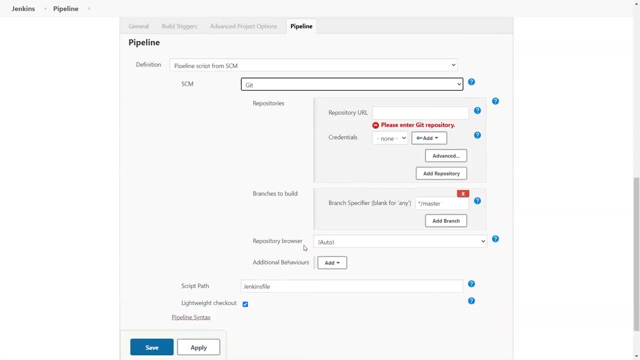 then go with the git here. now in there the jenkins file is the name of the file, of the pipeline's script, and i'm going to put my repository over here in this one. now this repository is of my git, which is like having a maven build pipeline which is available there. it's having some steps related. 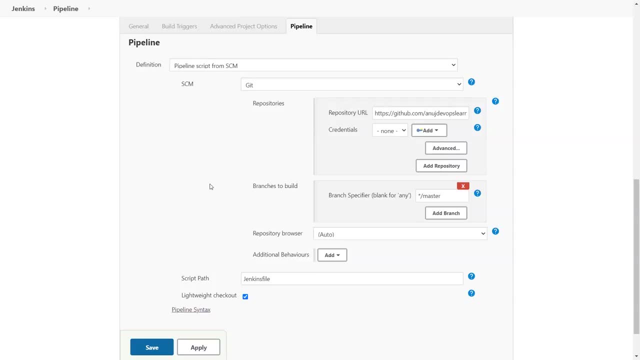 to ci with for the build and deployments and that's what we can follow as such over here. now, in this one, the uh. if it is a private repository, definitely you can add on your credentials, but this is a public repository, a personal repository, so i don't have to put any. 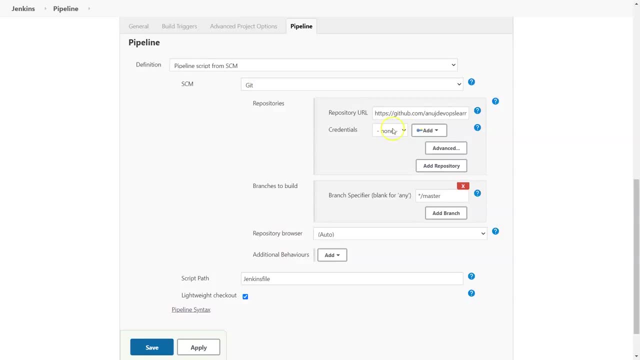 kind of credentials, but you can always add the credentials with the help of add here and that can help you to. you know, set up, whatever the credentials, the private repositories you want to configure now. once you save the configuration here now what it's going to do is that you- it's 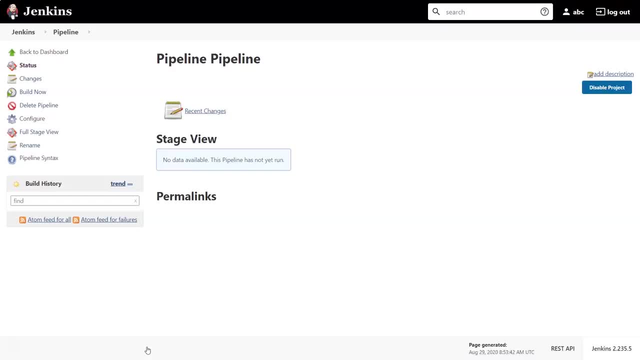 going to give you a particular page related to build now. if you want to run, if you want to delete the pipeline, if you want to reconfigure the pipeline, all these different options are available there. so we are going to click on the build now, here and when. i do that immediately- the pipeline. 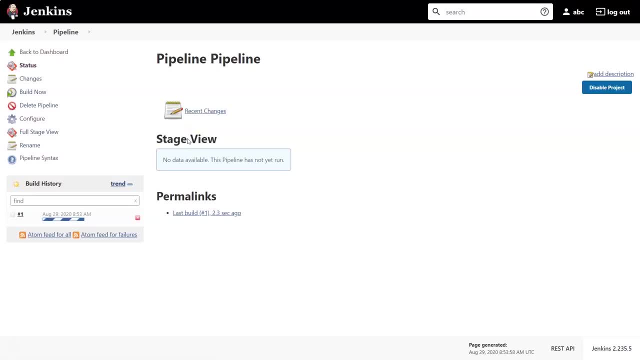 will be downloaded and will be processed now. you may not be able to get the complete stage view as of now because it's still running. so, yeah, you can see that the checkout code is done. then it's going on to the build. okay, that's one of these step which is there now, once the build will be done. 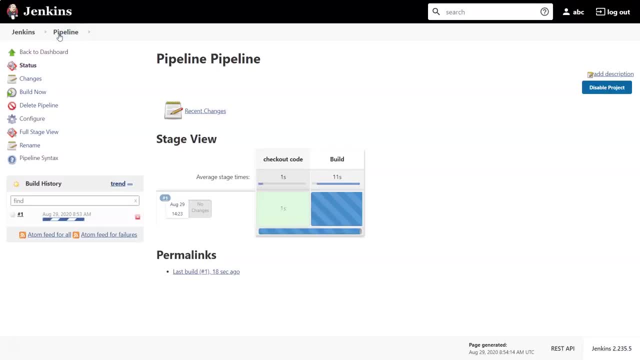 so it will continue with the next steps, with the next for the steps there. so you can also go to the console output log here, like you can click on this, or you can click on the console output to check the complete log which is happening there. in fact, you can also see the stage wise logs also. uh, because that is also very important when you. 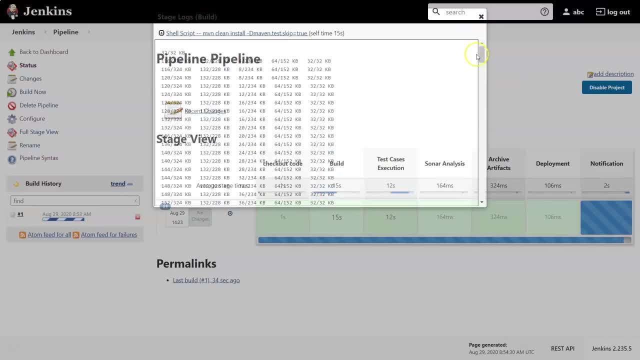 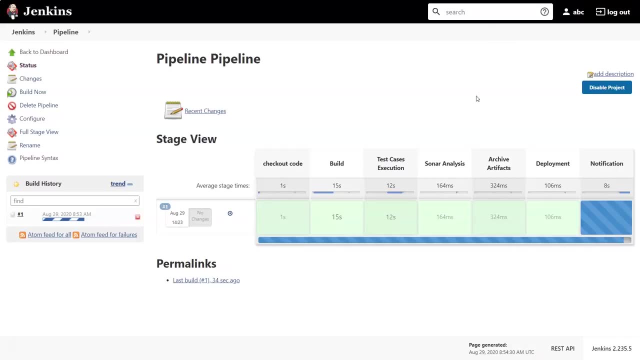 go for the complete logs. uh, it may. you know uh have a lot of steps involved and you know a lot of logs will be available there. but if you want to see a specific log of a specific stage, that's where this comes into the picture and, as you can see, that all the different uh steps, like test cases, 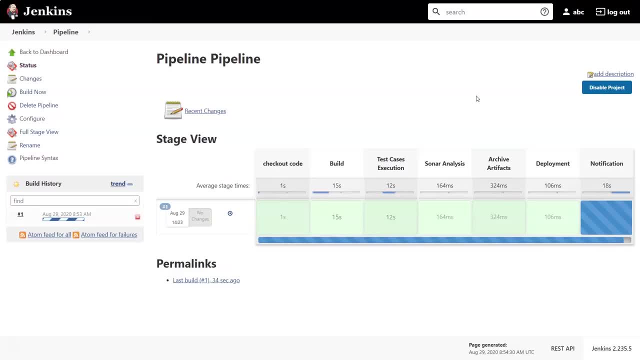 executions, the snarkube analysis, the archive artifacts, deployment and, in fact, the notification. so all this is a part of the build. so you can see that all the different uh steps, like test cases, etc. and that's what i am sharing with you here in this particular, this whole pipeline is done here. 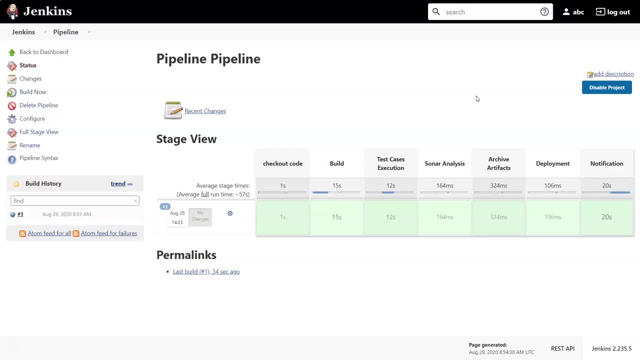 and uh, you know, you get a kind of a stage view its success over here and the artifacts is also available to download so you can download. this war file is a web applications as such over here. so this is what a typical pipeline looks like. that how the automation, the complete automations.